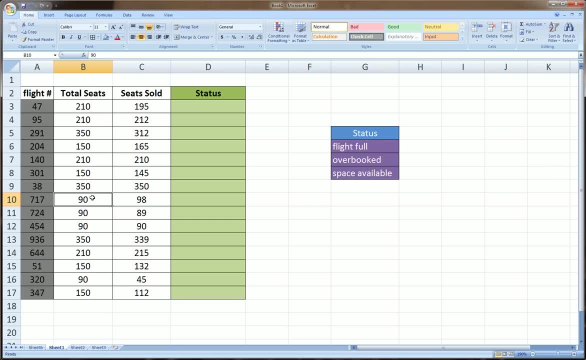 So I just went off the presumption that there's four types of aircraft and these are the four capacities. Okay, here are the seats sold. So, as we know, sometimes airlines oversell seats and they have all different kinds of ways of dealing with things like that. But here we're going on the assumption that they can oversell a flight, and obviously they can undersell a flight, like in this case. They sold less seats than the number of seats on the plane and also they can fully book a flight. 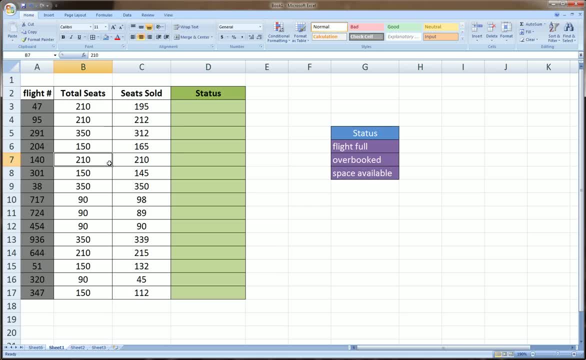 Which is a case like this where there's 210 seats and there was also 210 seats sold. okay, And basically what we want in this column is the status of the flight. So- and here I just put a little note on the side here- and these are the three statuses or stati that we'll consider. 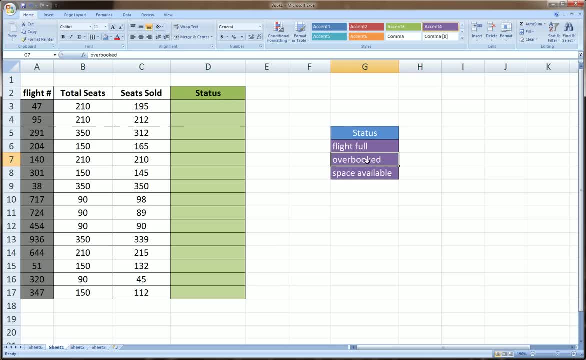 The flight is full. the flight is overbooked, meaning we sold more seats than there is. There's space available, and space available would be like the first example here: There is 210 seats and we only sold 195.. Okay, so there's three possibilities for each one of these flights. 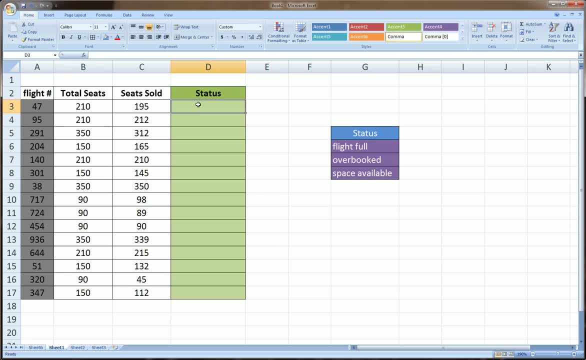 And, as we know, because you know, if you're new to If Functions, maybe you should go and watch my earlier If Function tutorial on my channel As a primer for this. but, as we know, an If Function has three parts. 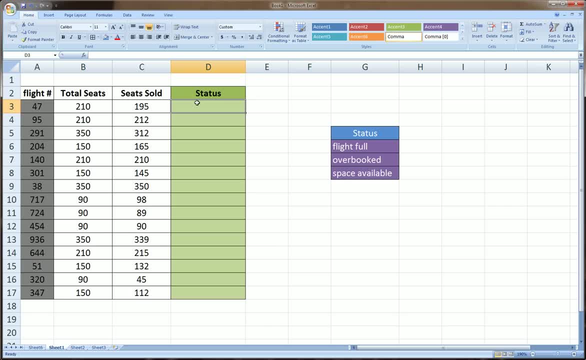 One is the test, and the second and third part are the values returned. if the test is true and if the test is false, So it could give you back two things right, Either or, Whereas here we have three possibilities. So here you're going to use nested If Functions okay. 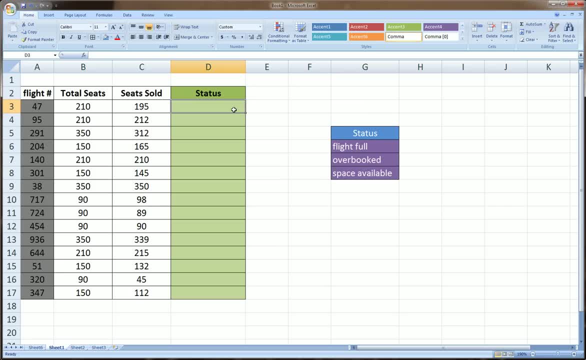 So let's get started. Since we're all pretty familiar with If Functions, we know we start with equals If and the first argument is the logical test. So, arbitrarily, I'm going to choose to make the first test: whether the flight is full. 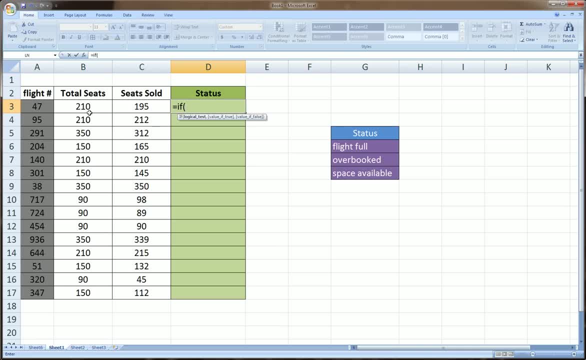 So treating each row independently. let's deal with row one Does. how can we test whether the flight is full? Basically, that means if cell B3 equals cell C3, right. If B3 does not equal, then the flight is full. 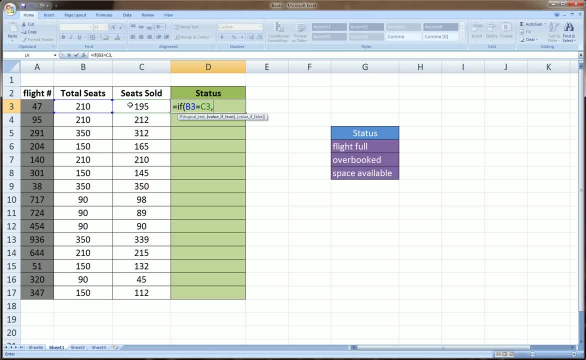 So that's the first test comma. What do we want Excel to return if the flight is full, Or in other words, if this test, this first test, is true, Well, obviously we want it to return in quotes: flight full right. 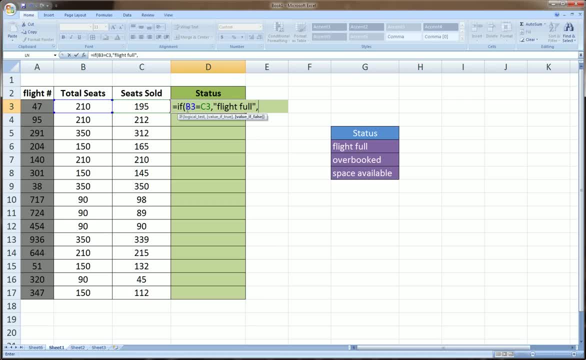 Comma. What do we want Excel to return if B3 does not equal C3? Or, In other words, if this test fails? And what we want it to return if this test fails, is either of two things: Either it's overbooked or there's space available. 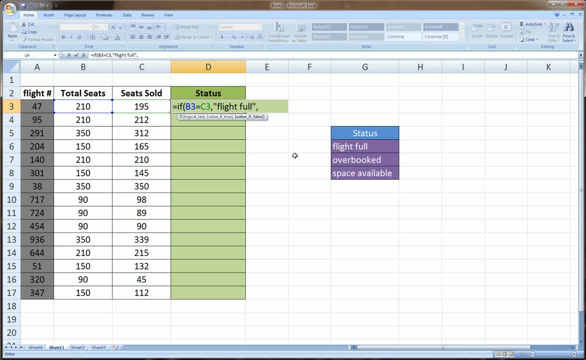 So we can't just write overbooked here, because there's also the possibility that there's space available. So this is where a nested If function will come in. So basically what's going on here is: if this test is true, then we get, then Excel will. 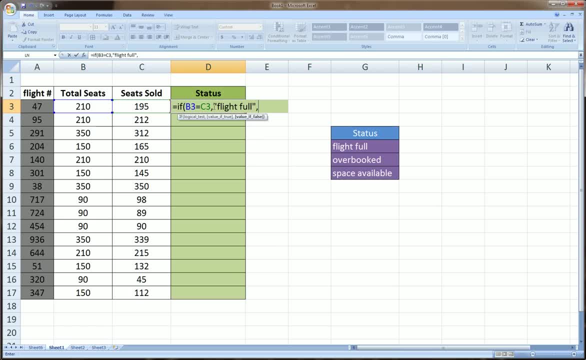 return flight full and we're done. Comma. If this test is false, we will continue with another If function, another test. So we type If here. So it'll only get this far to the second If if this test fails, Because if it's true we end with flight full and Excel doesn't continue any further on. 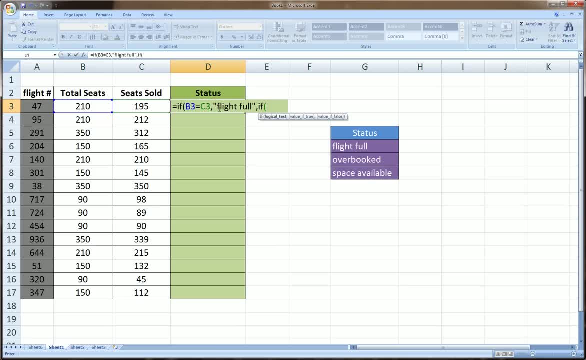 this function. Okay. So now, If this test fails? Now What's another thing we want to test? Obviously, let's just take it in the next order. We want to test if it's overbooked. How do we test if this flight is overbooked? 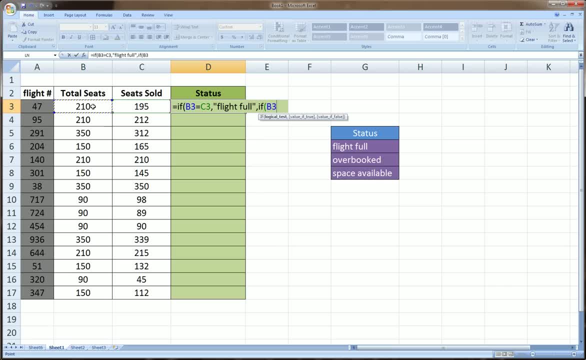 We can see if the total seats is less than the seats sold, Because if the total seats is less than the seats sold, then we've overbooked the flight, Right? Okay? And if this is true, of course, this will be overbooked, right. 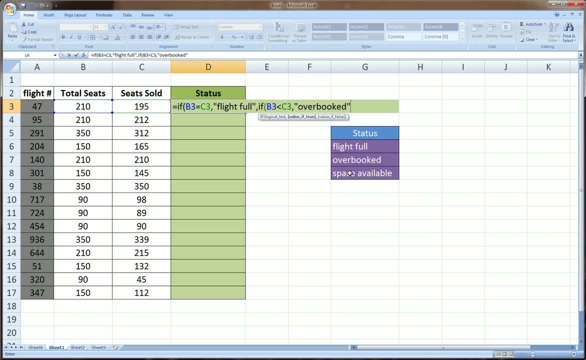 And then, if we think about it, there's only one other possibility, and that is that space is available, And space is available will occur when total seats is greater than the seats sold. But we don't have to test that because by default, that's the only thing left. 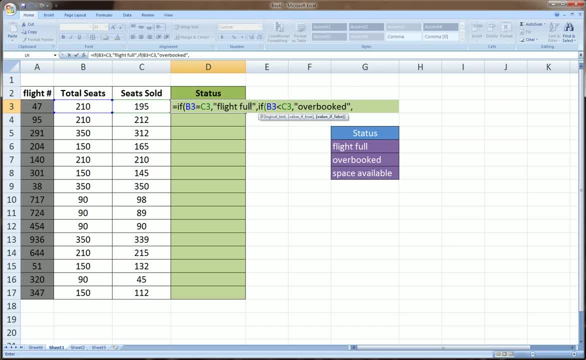 In other words, If this test fails And they're not full, then Excel will go to this test, And if this test fails, then it's not overbooked, then there's only one other thing it can be, And there we can just type space available in quotes. 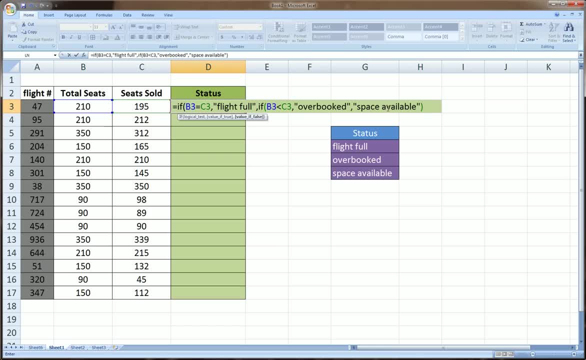 And we'd close the parentheses on the nested if function And then close the parentheses on the larger if function that's containing this nested if function. And remember the open parentheses have to equal the closed parentheses And this becomes something that gets quite annoying when you have five or six if functions. 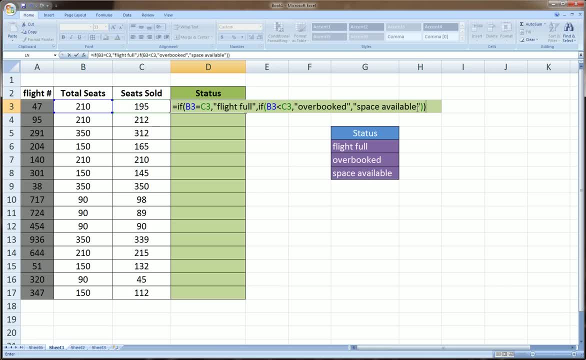 nested within each other, But over here it's clear There's two open and two closed. Okay, So let's just review this function again before we hit enter. So this is what's going on. First, The if function is testing. 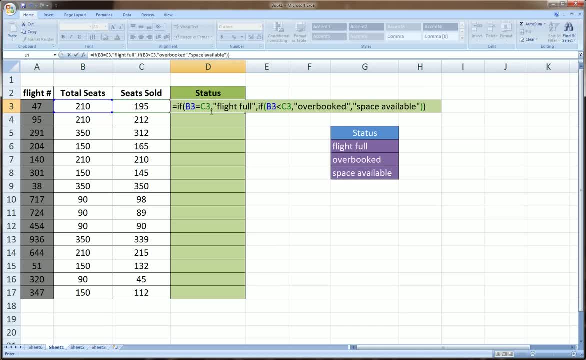 Whether B3 is open or closed If B3 equals C3. If they equal each other, then the flight is full And we're done. Excel will stop right there and chop it off right there. But if B3 doesn't equal C3, then Excel will continue. 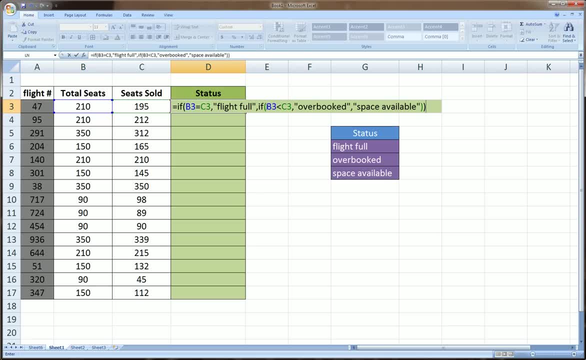 And it will go into another if function, And this time it will test if B3 is less than C3. And that would mean that the flight is overbooked And it'll return open, Overbooked, Overbooked. 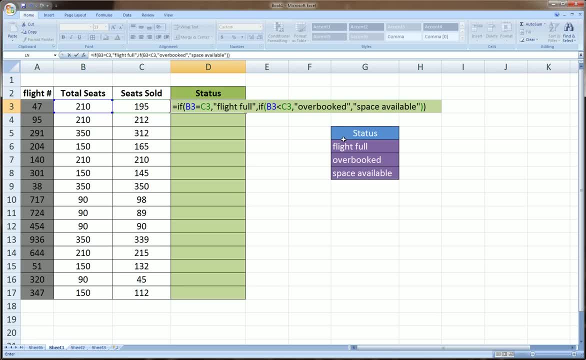 And it would finish there if that was the case. But if this fails and this fails, then there's only one thing left, And that is the final status, which is space available. Now we hit enter And in this first case, before we hit enter, I always like to take a little guess at what. 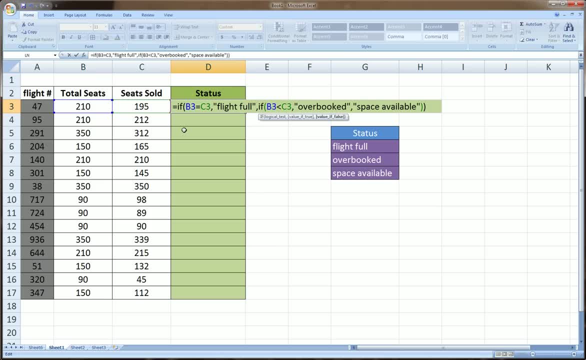 it's going to be And obviously in this case there's going to be space available. So let's see: Is this the right thing? And voila, it does. And just like all functions, if it's done correctly, we can drag it down. 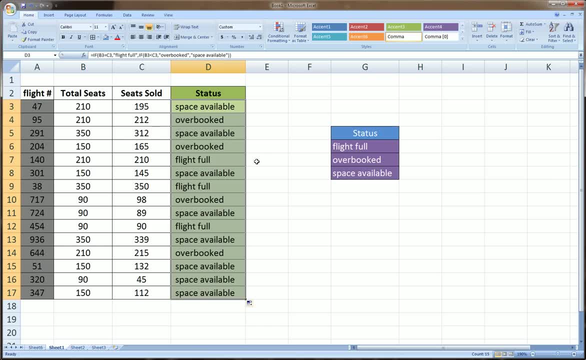 Let's drag this all the way down and go through a couple of rows to see that it worked properly. The second row: there's 210 seats And we sold more seats than we had, So it's overbooked. Makes sense.